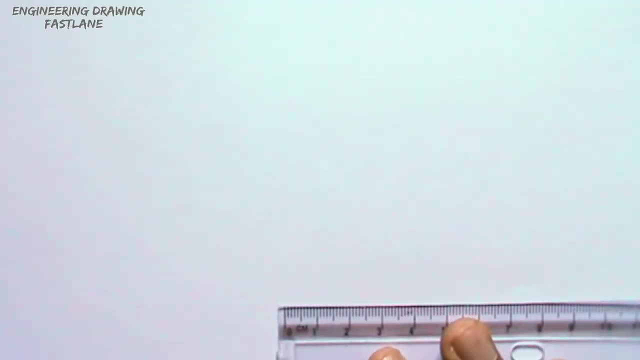 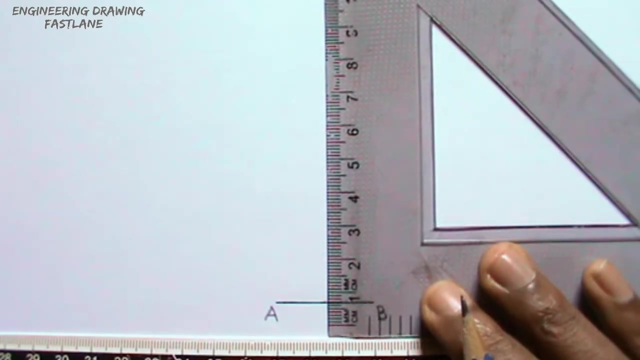 Welcome To draw any regular polygon, given the length of the side. the first step is to draw a horizontal line and label it. I have already done this step. The next step is to draw a vertical line to divide line AB into two equal parts. 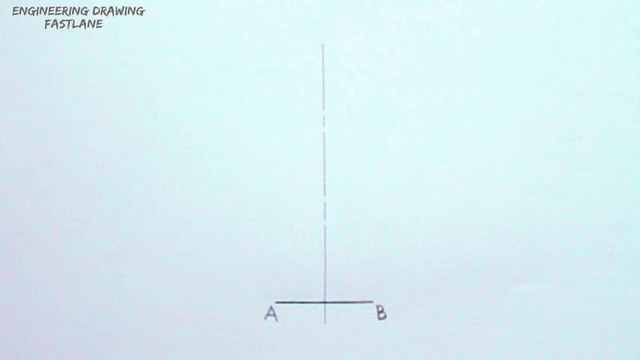 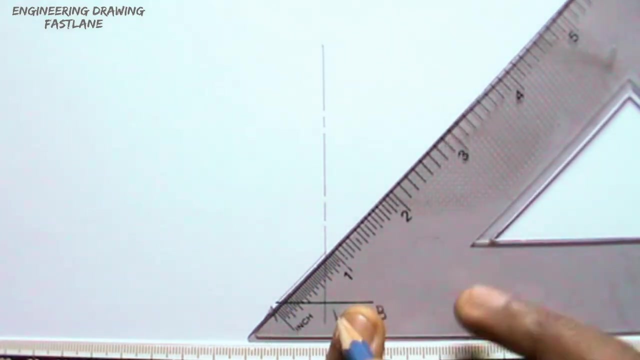 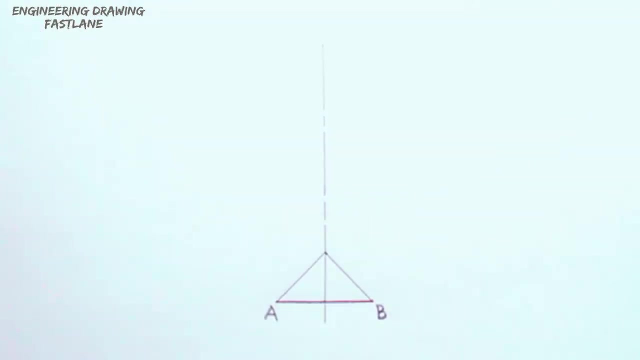 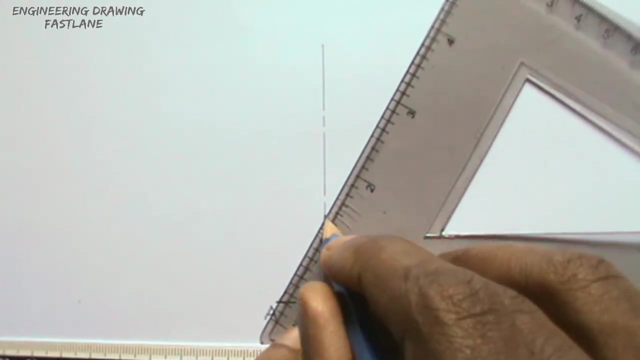 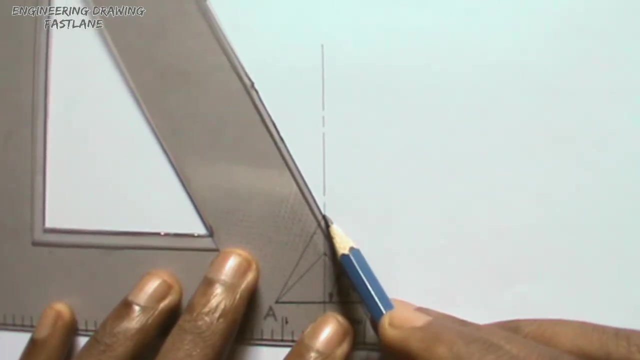 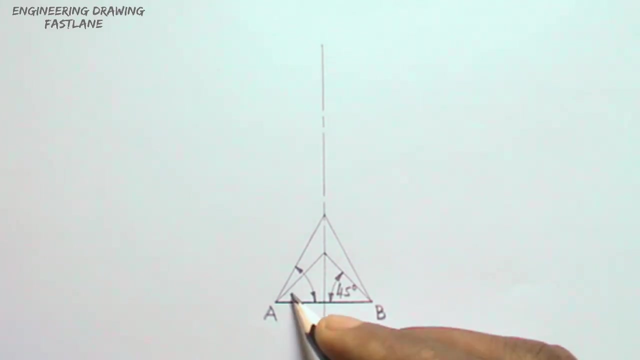 Next, draw a triangle with base angle 45 degree on line AB. Draw another triangle with base angle 60 degree on line AB. Draw another triangle with base angle 60 degree on line AB. Number the apices of these triangles: 4 and 6.. 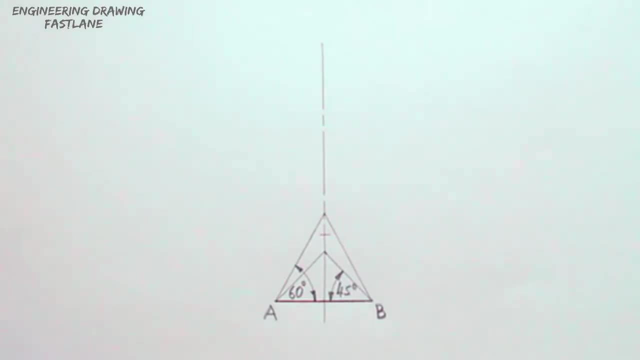 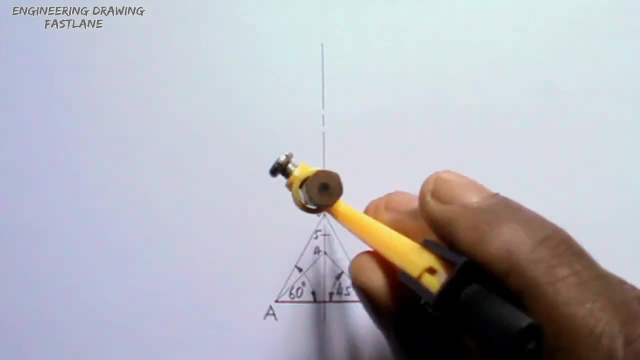 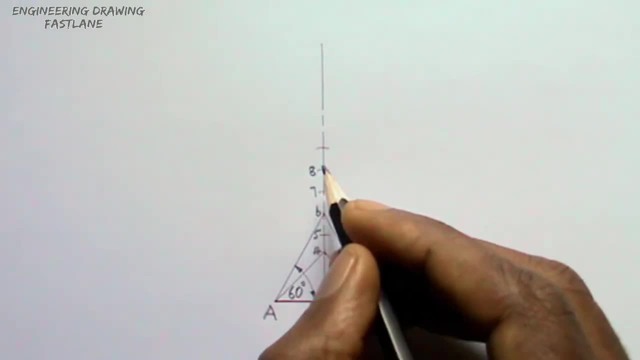 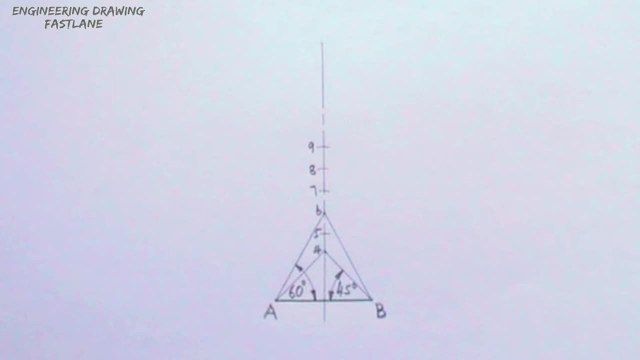 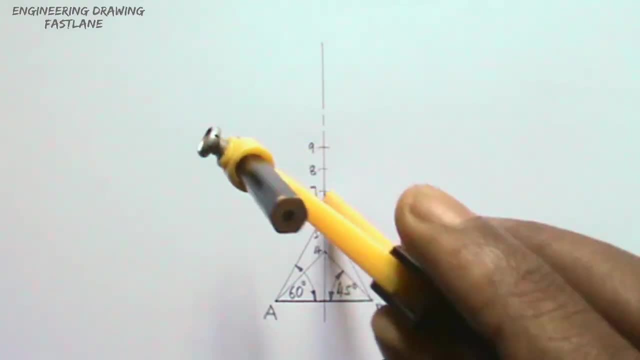 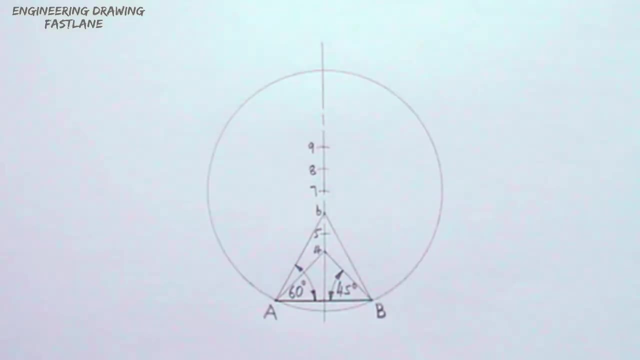 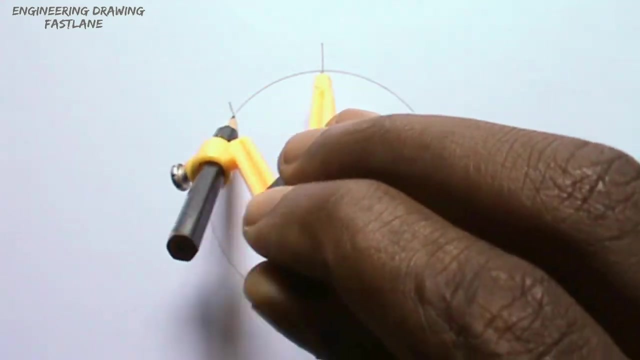 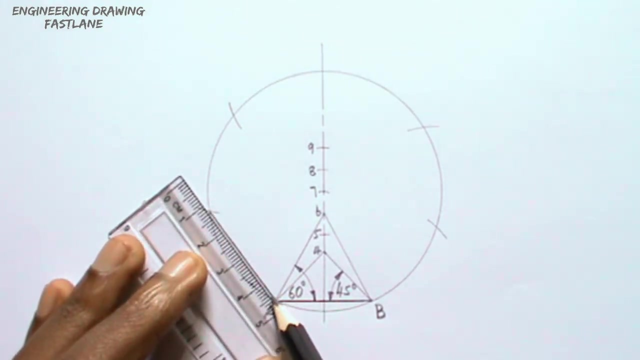 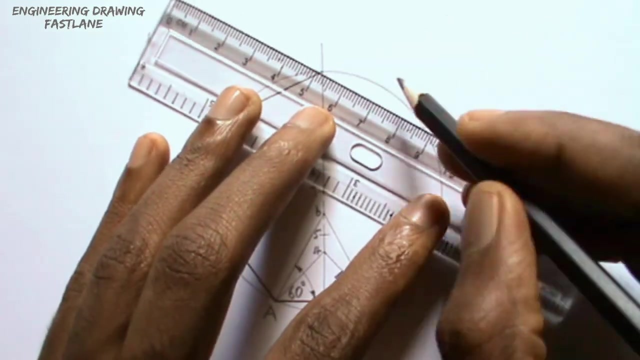 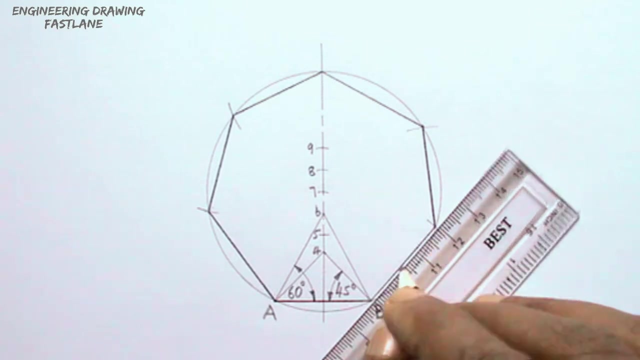 Mark off three more points from 4. Place my compass on point 7, because I want to draw a heptagon With radius AB, I will use my compass to step round the circle. I will now join the point to obtain my required polygon, which is heptagon.